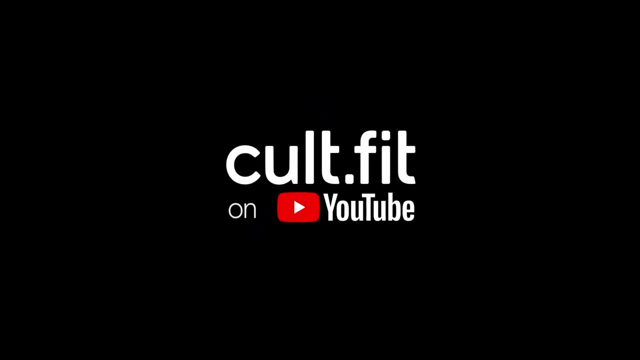 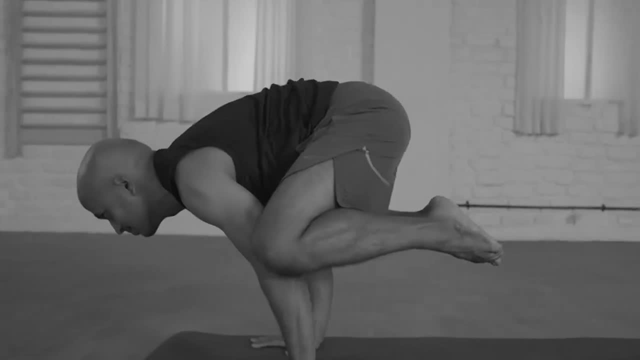 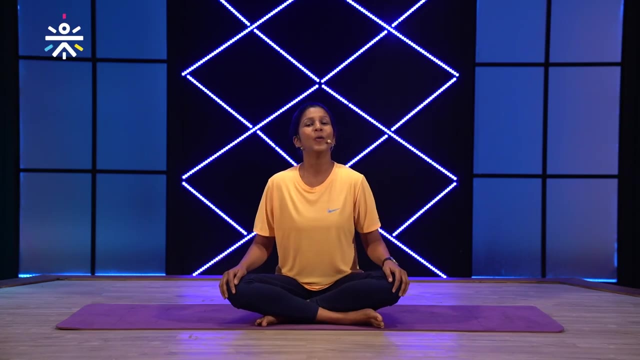 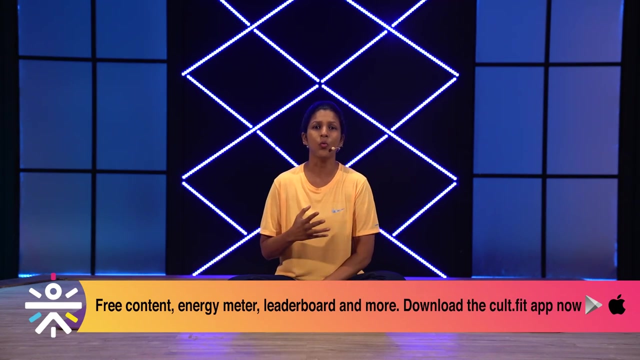 Welcome everyone and namaste Welcome to another quick and easy yoga session with me, Divya Rola. Today, our focus will be on heart health and the asanas and the pranayamas that will be beneficial to the heart. Now, yoga approaches heart health in two different ways. One is obviously to increase cardiovascular endurance. 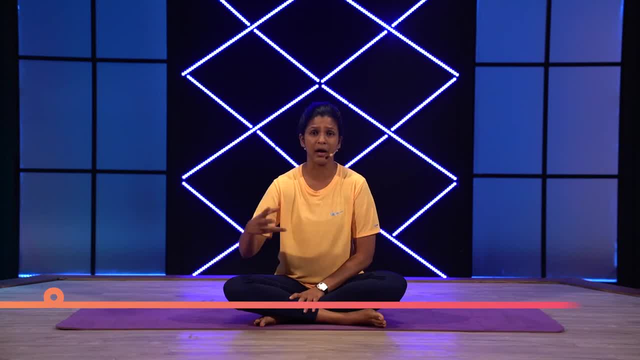 So things that will increase the rate of the heart. and two is to help the heart rest and send a lot of blood flow to the heart, So all inversions where the hips are higher than the chest. One: it increases the size of the heart because a lot of blood goes into the heart and it also hence works the muscles of the heart. 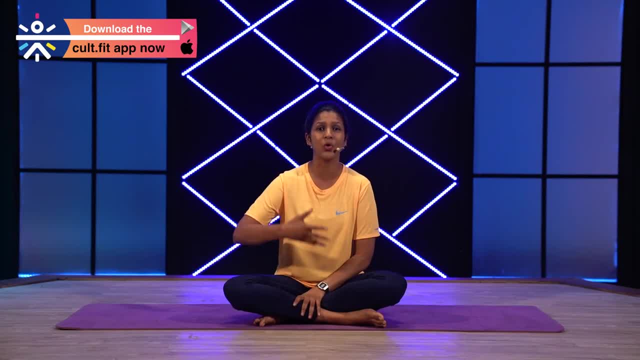 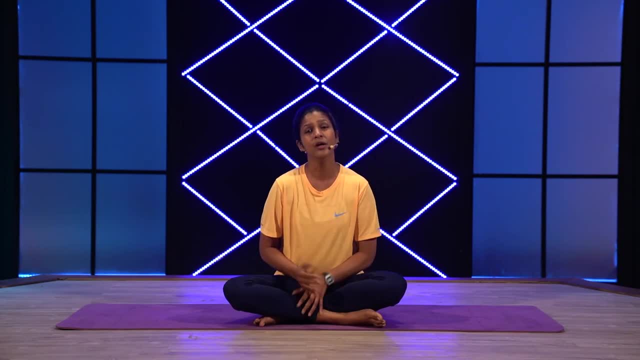 Two, it allows the heart to rest, because the heart is no longer having to work against gravity to pump the blood from our feet all the way back up. So with that, let's get started with a quick warm up. Now, sitting up tall, We are going to sit with our legs crossed, shoulders roll back and down. 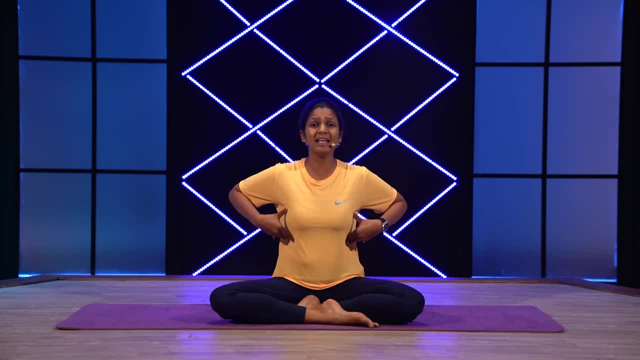 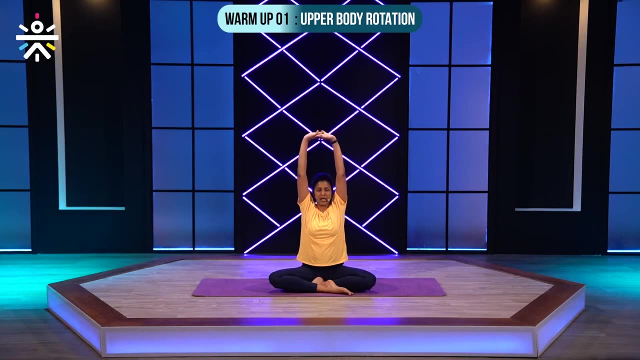 Now, everything that we do today will help in increasing our thoracic cavity, So increasing a lot of space where the heart is. So, shoulders, roll back, sit up tall Now as you inhale. lengthen the arms up, interlock the fingers and stretch the arms. 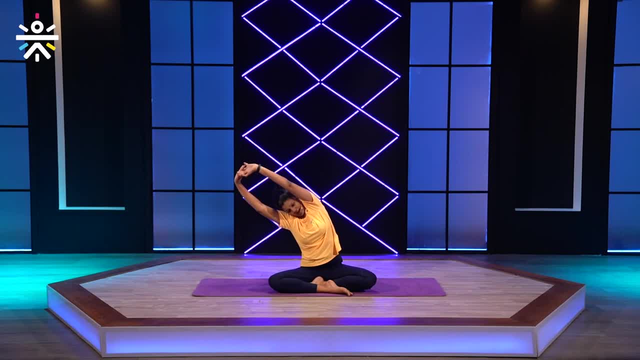 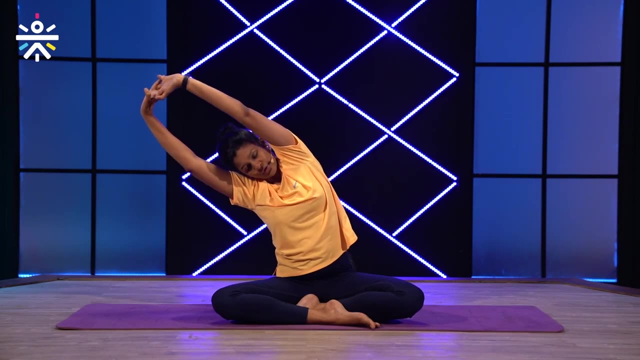 From here, inhale to the right side, Exhale back down, Inhale to the left side and coming back up. So let's do this together: As you inhale to the right, go all the way down without bending the elbows. 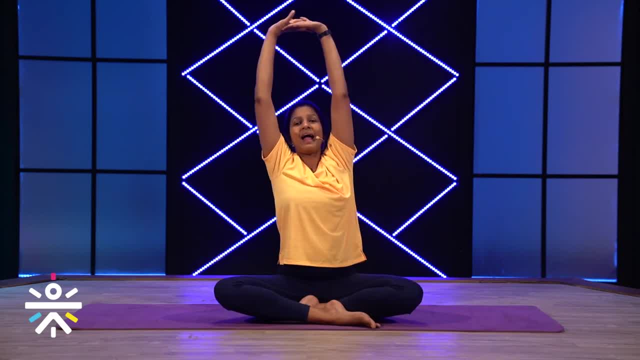 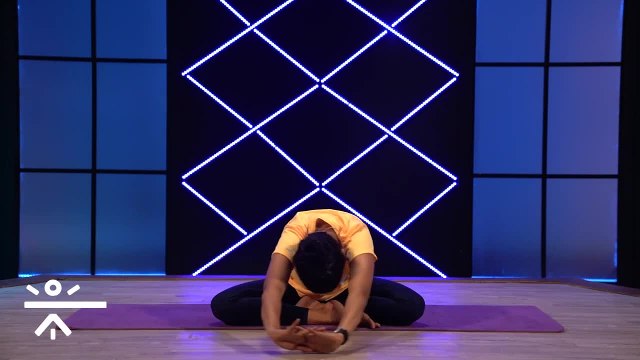 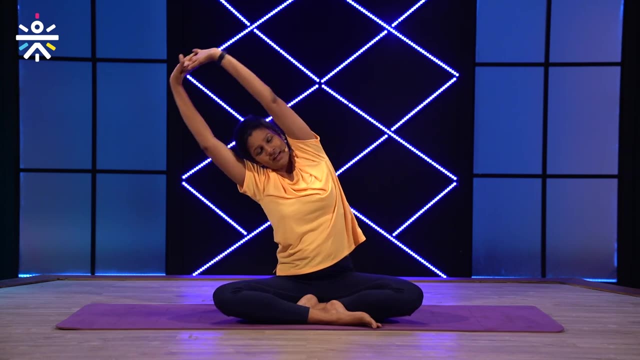 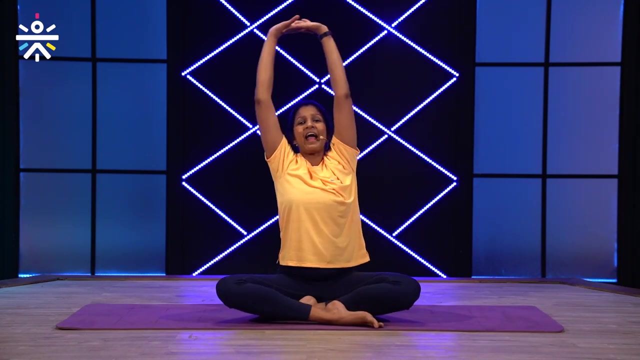 Inhale to the left and exhale coming back up. Inhale right, exhale down. Inhale open to the left, exhale back up. Try not bending the elbows To the right all the way down To the left and coming back up. 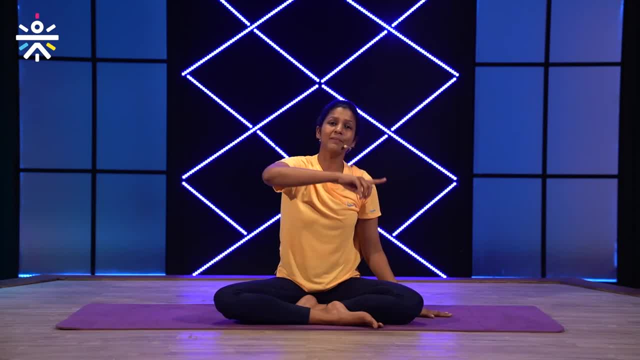 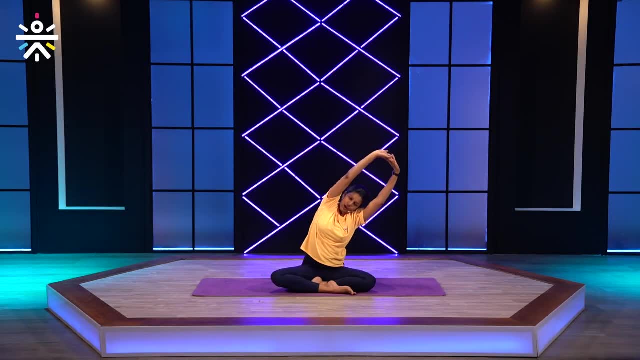 Release the arms, take a breather. We will do the same thing on the opposite direction. So inhale, lengthen the arms all the way up. Now reach to the left, Lengthening the right side of the body. Come all the way down. 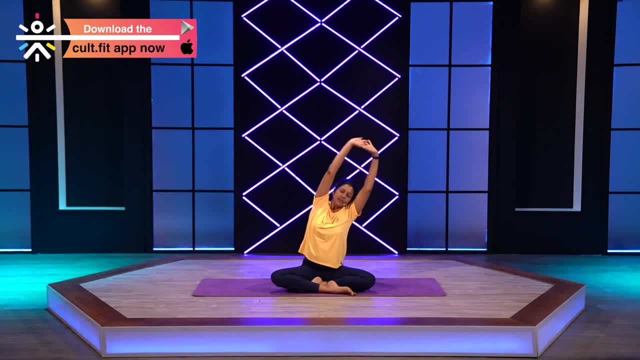 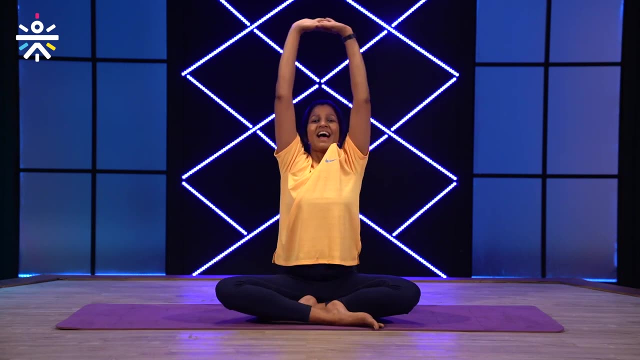 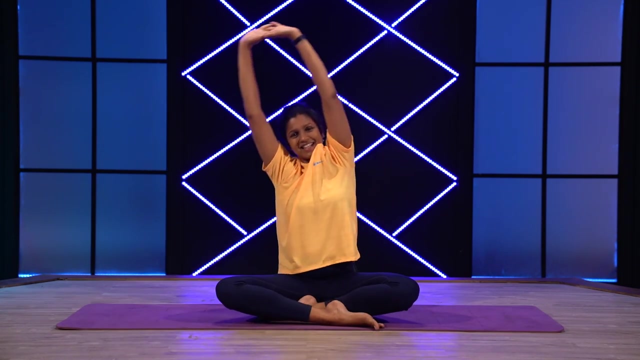 Reach to the right and come back up To the left all the way down To the right and back up Left and down Right and back up Left and down Right and back up Exhale. slowly, release the arms. 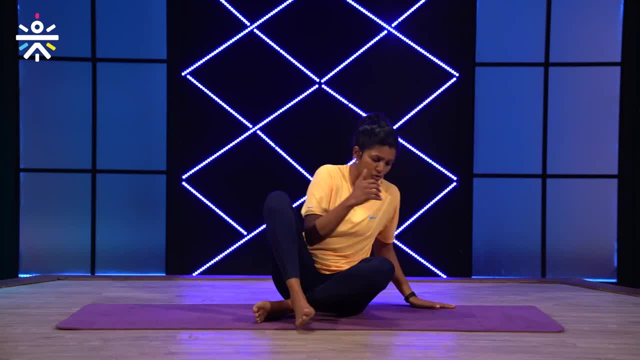 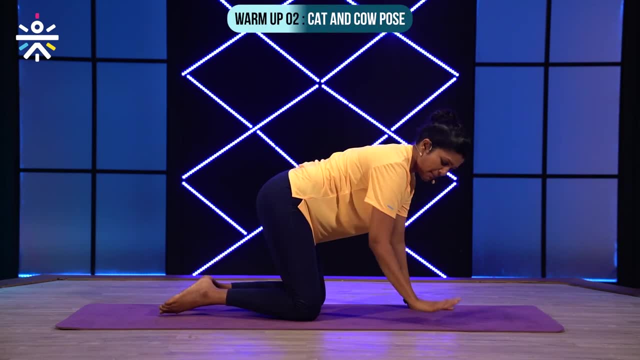 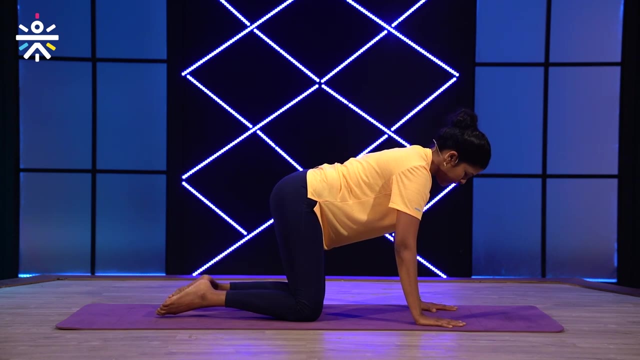 Excellent. Next, moving on everyone, come on to all fours with me. We will do some cat and cow. So making sure that your palms are directly under the shoulders, Your knees are directly under the hips, Feet are flat With my breath, inhale, arch the spine. 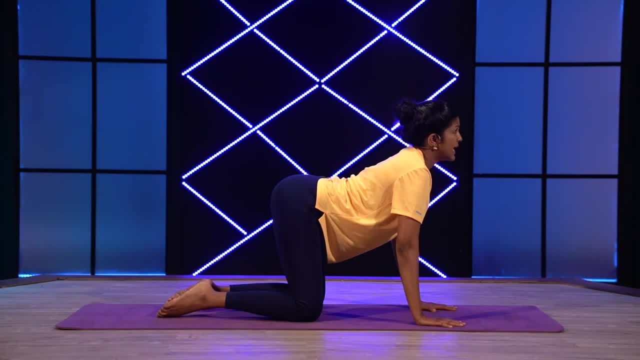 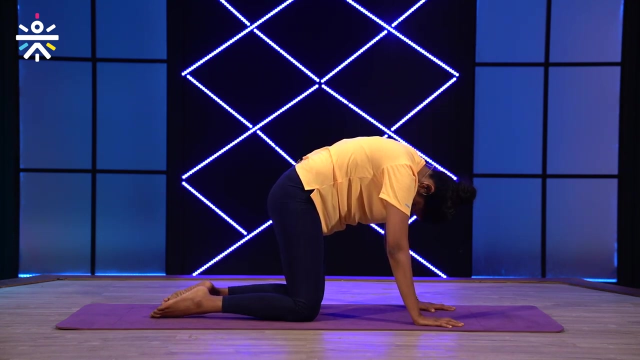 Chin up, Try not bending the elbows. Exhale- push into the palms. rounding the spine. Inhale and arch. Exhale. draw the navel in rounding the spine. Inhale and arch. Exhale. draw the navel in rounding. 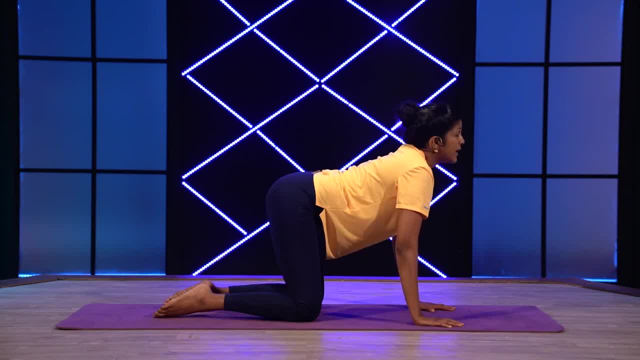 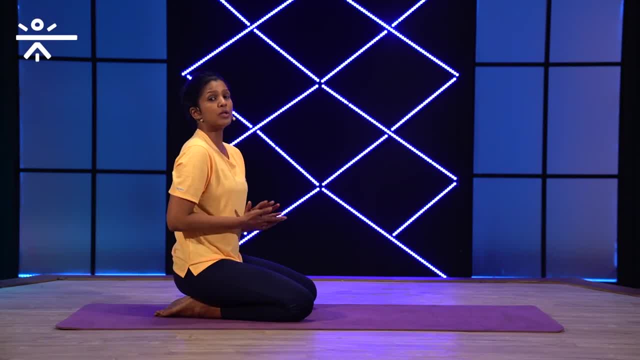 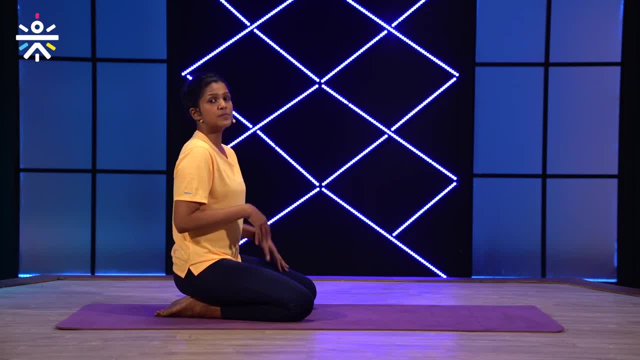 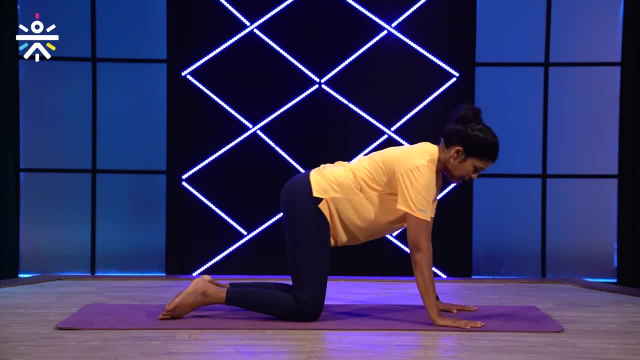 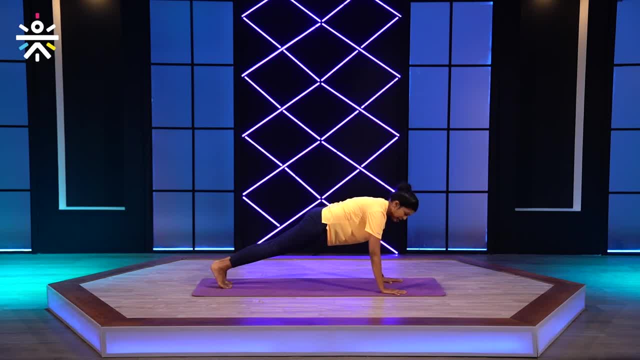 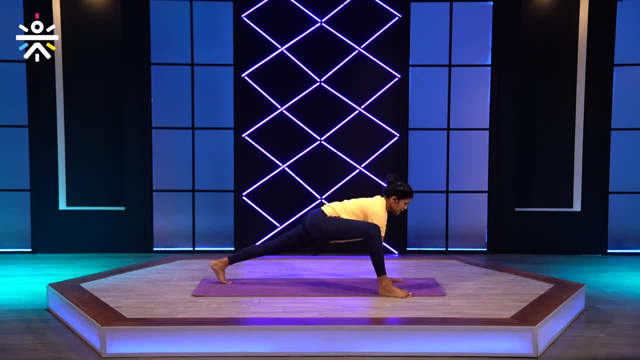 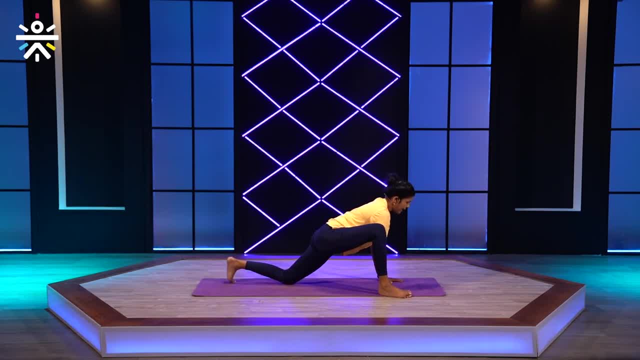 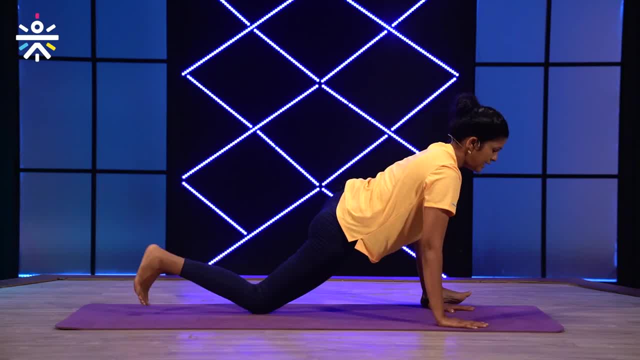 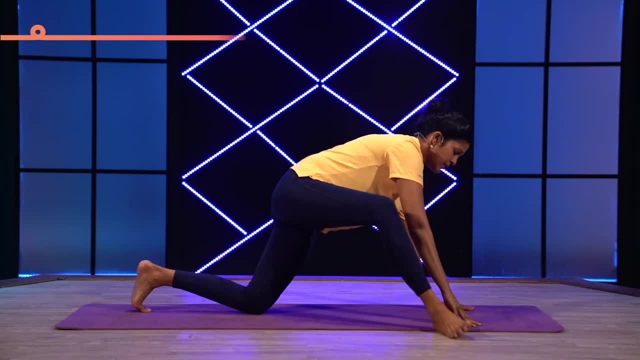 Exhale. draw the navel in rounding, Inhale and arch Exhale. draw the navel in rounding left leg back, right forward, and we'll do this five times on each side together. so get ready. palms under the hip, palms under the shoulders, knees under the hips. 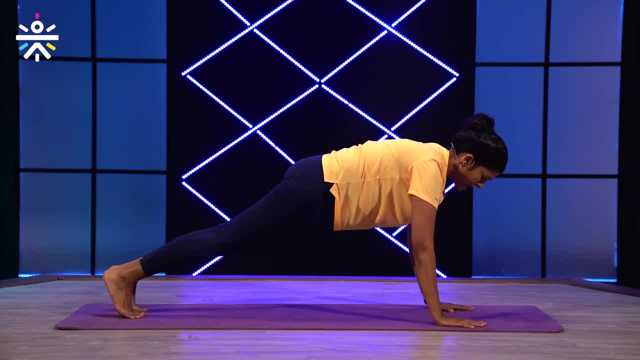 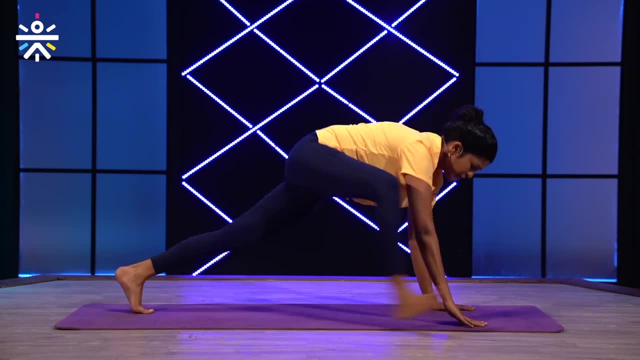 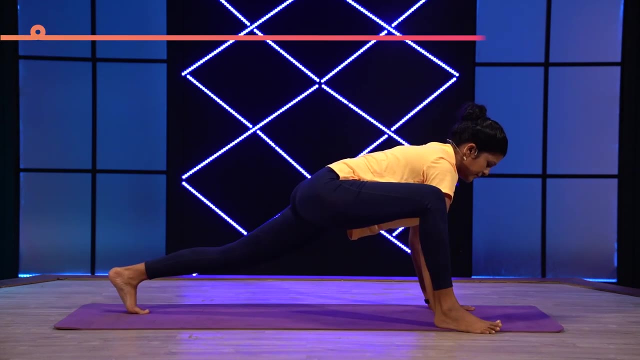 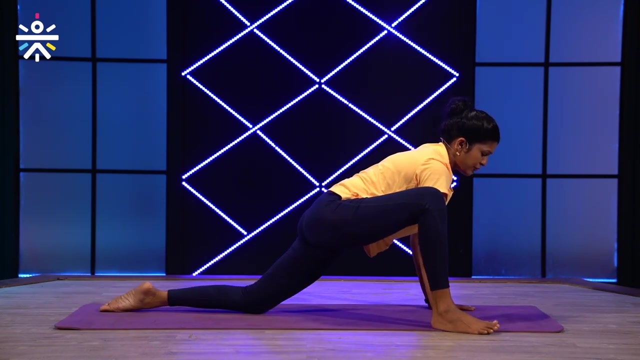 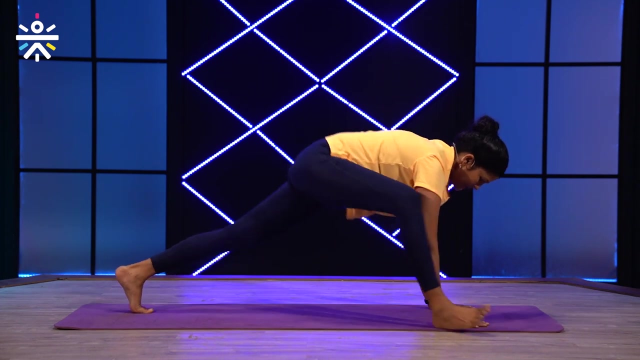 now everyone get into a plank position from here: right forward and back, left forward, back right, drop the hips and left on three, and on the left side on four, you can drop the knee down if you want, and left on five and left. let's just do this one more time. six: 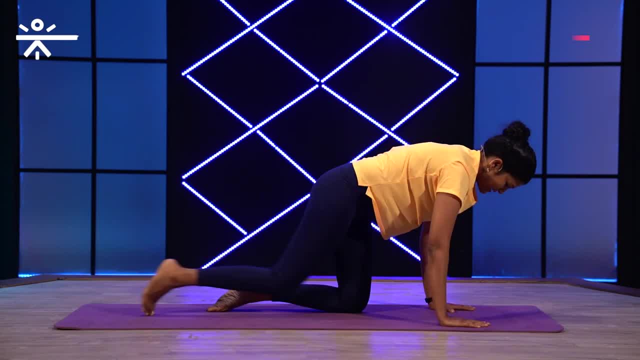 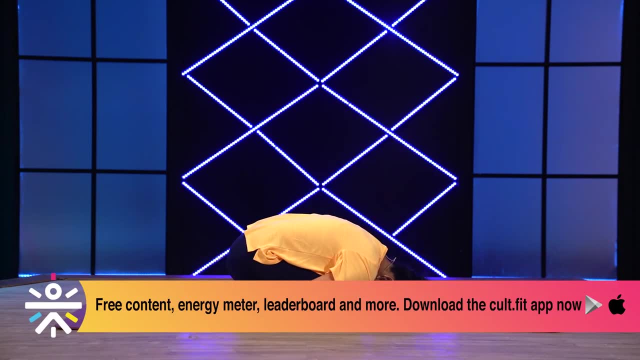 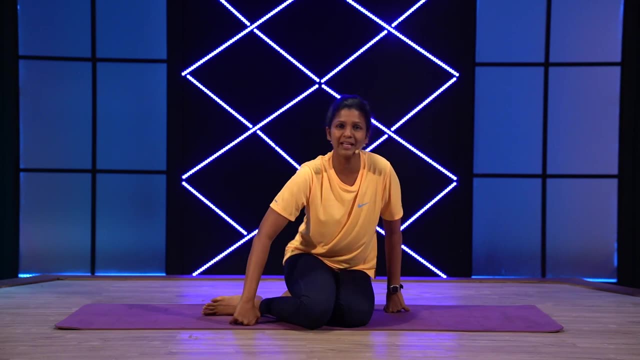 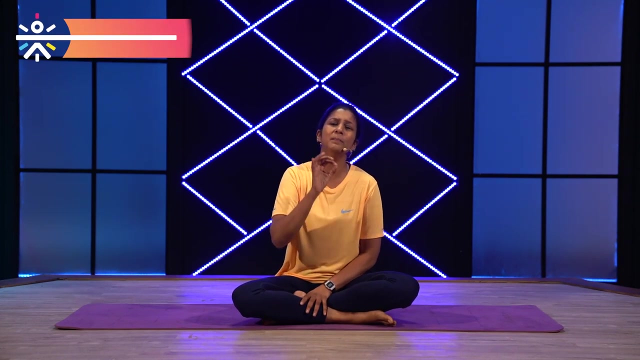 and left, take the leg back, drop the knees, drop the hips and everyone relax in child's pose. now, while you're relaxing, quickly looking at the next posture. now, the next thing that we are going to do is a simple inversion, an inversion that most of us will be able to do comfortably. 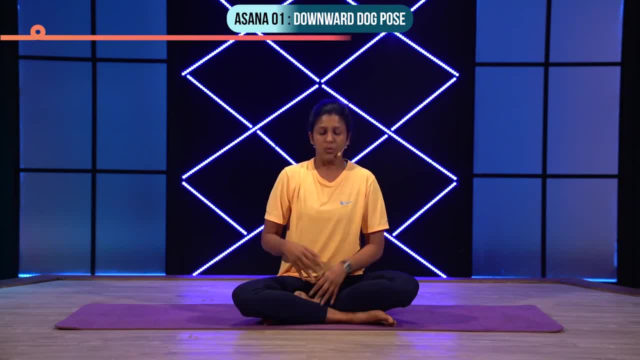 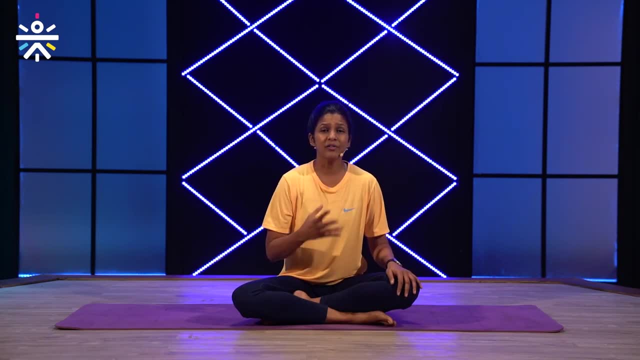 which is the downward dog position. now, when our hips are above the chest, a lot of blood flow goes to the heart, so inversions are excellent for the heart, but inversions like headstand or shoulder stand may be challenging for some of us, so we're going to pick up very simple and effective inversion. so 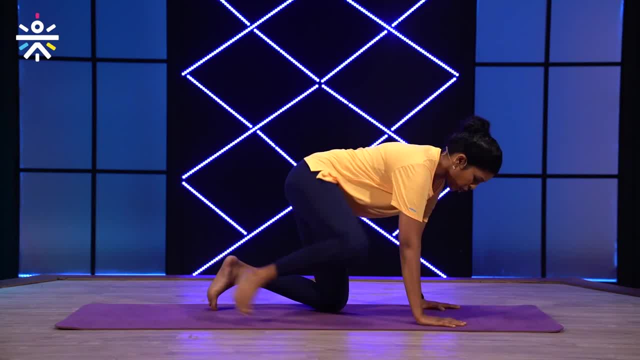 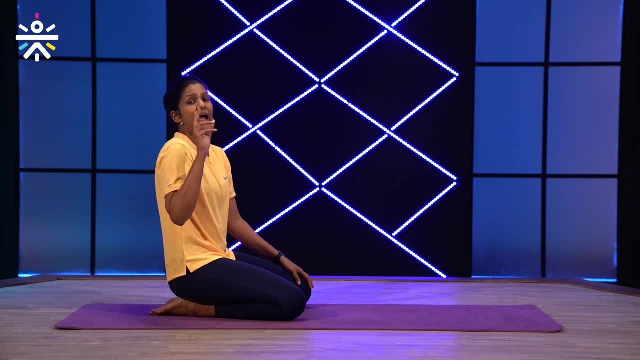 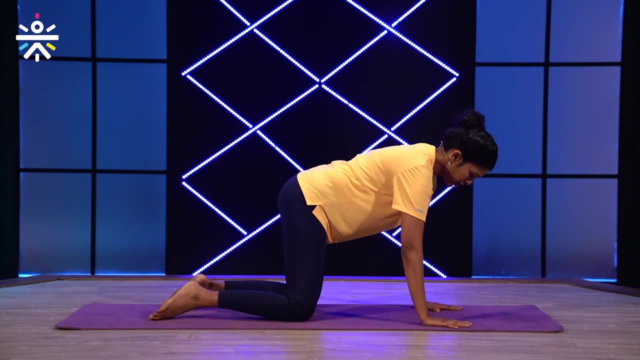 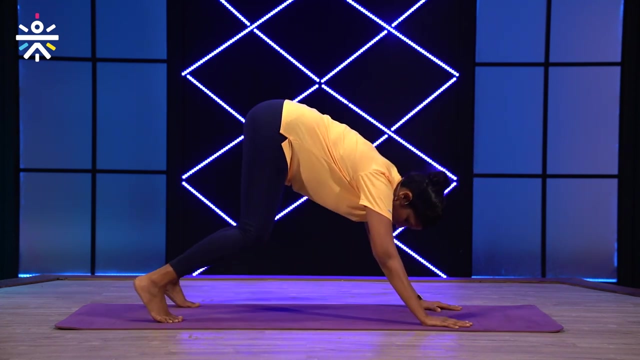 together with me. now, coming back on to all fours, this also we're going to do dynamically for the first three times and then we're going to, in the last time, hold and hold for ten counts together. so palms are under the shoulders, knees are under the hips together, tuck the toes everyone and lift the hips up, keeping. 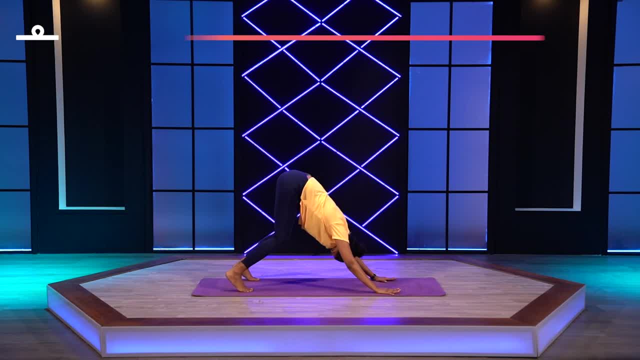 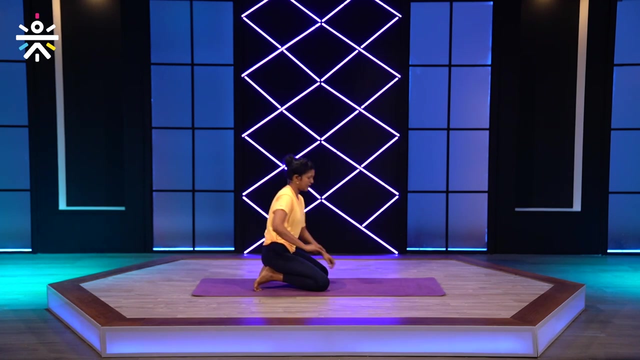 the knees bent and hold here and dropping back down together again. tuck the toes, spread the fingers shoulders away from the ears and just lift the hips up. knees are bent and dropping back down now the last time. we're now going to hold it for 10 counts, so, together with me holding the downward, 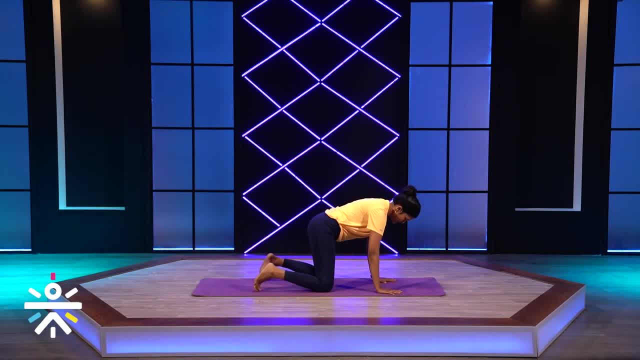 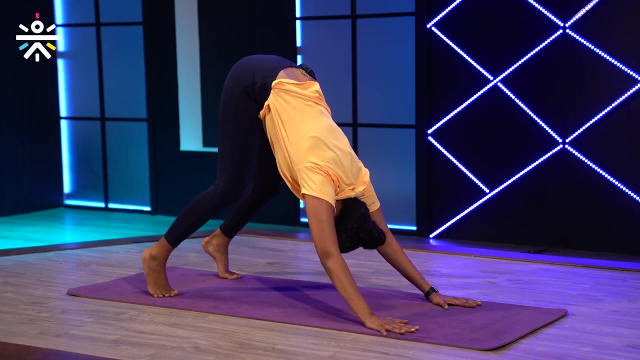 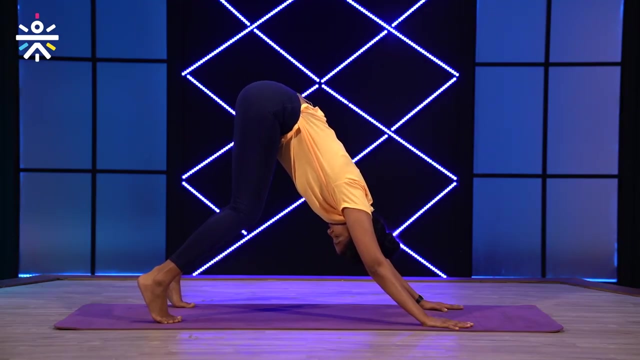 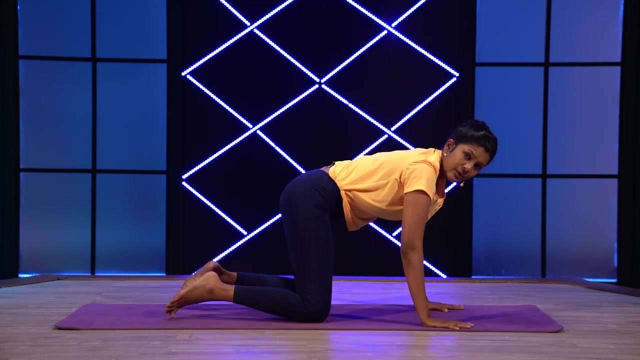 dog position modified for 10 counts. duck the toes and lift the hips up. now really Bend the Knees, Lif, Lif, heels up and try and bring the chest closer to the thighs, Holding here on 1,2,3,4,5.. Keep pushing into the palms chest towards the thighs 8,9 and 10.. Drop the knees down. 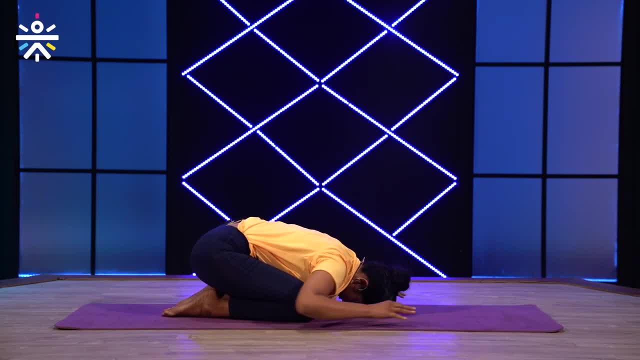 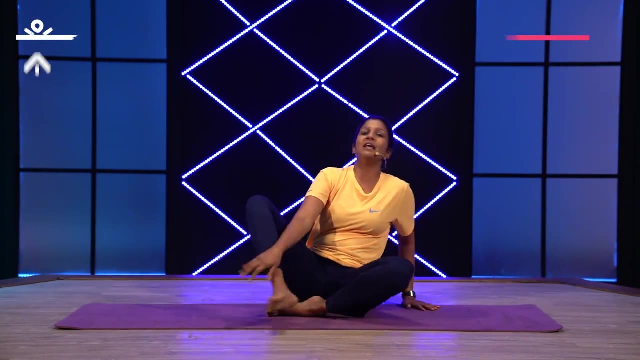 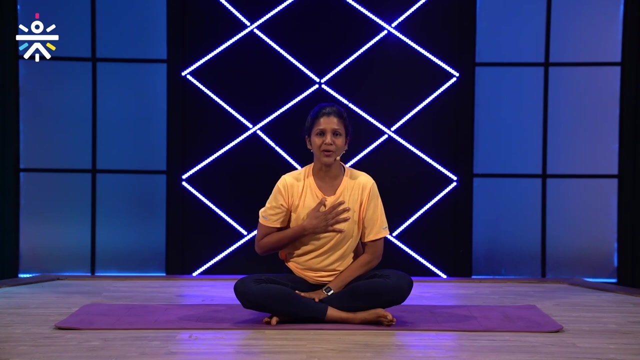 hips down and relax in child's pose, Slowly coming back up. Now, finally, we will finish with a pranayama. Now, this pranayama is wonderful for the body because this pranayama brings about a sense of balance both in the body and in the mind. 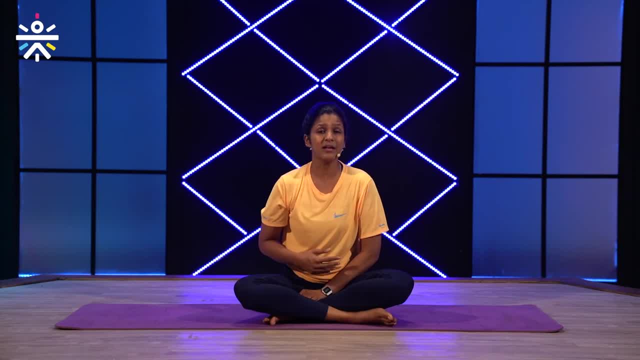 And this pranayama is also excellent for helping increase oxygenation throughout the body. Now for this anuloma viloma, or alternate nostril breathing, you will need to ensure that the right hand is in vishnu mudra like this, Closing the middle and index finger. Left hand remains. 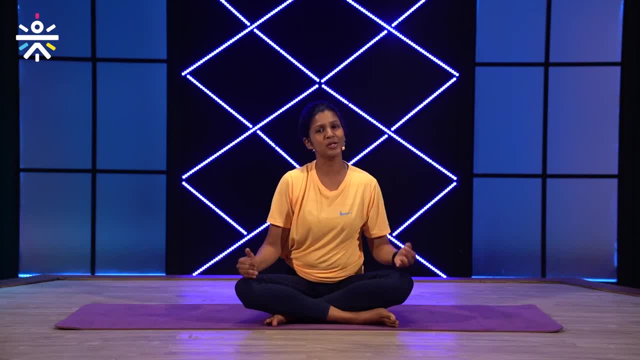 in chin mudra. While you are catching your breath, just watch me do a couple of rounds. So in this we use any one nostril to inhale and whichever nostril we are inhaling out of, we will exhale through the opposite nostril. And whichever nostril we exhale out of, we try and inhale. So the 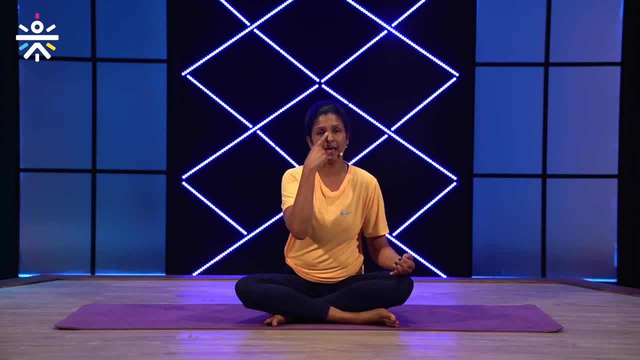 rhythm will be that inhale through the left, exhale through the right, inhale through the right and exhale through the left. This is one round of anuloma viloma And we will try to inhale for four and exhale for four counts. 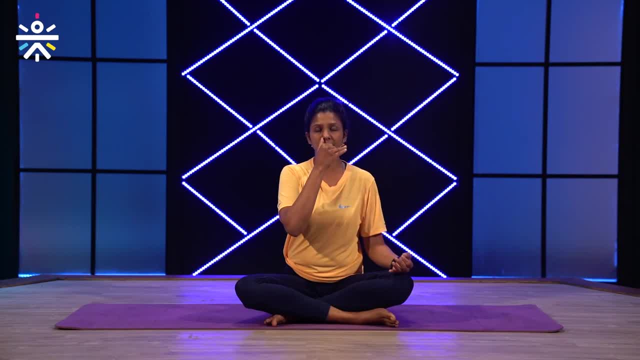 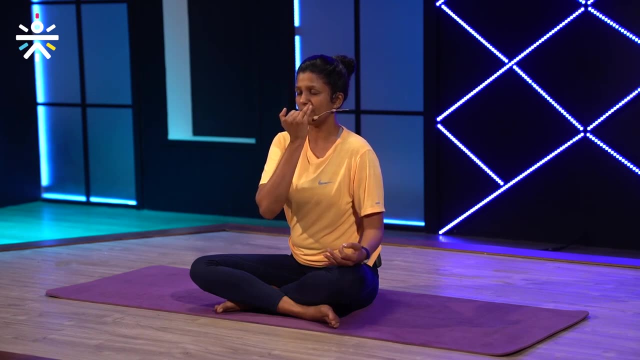 So, just watching round, one Inhale left, two, three, four. Exhale right, two, three. four. Inhale right, two, three, four. Exhale left, two, three and four. So let's get started. 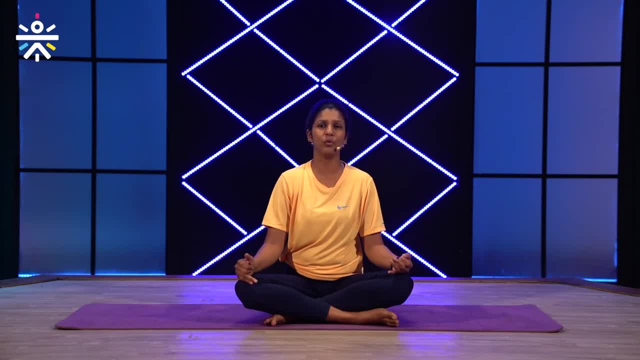 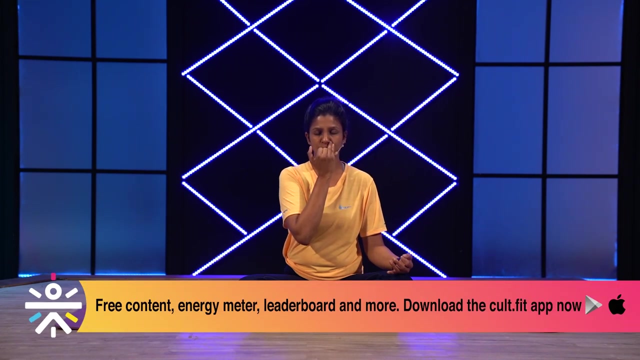 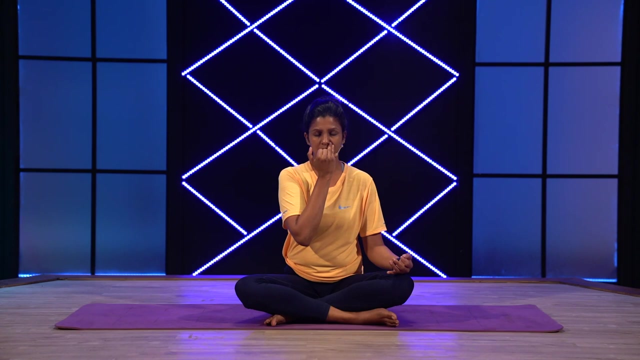 together We will do four to five rounds of anuloma viloma. Now, getting ready, Sit up, tall Eyes closed. Exhale completely through both nostrils and close the right nostril with the thumb. Inhale left, two, three, four. Exhale right, two, three and four. Inhale right, two, three.